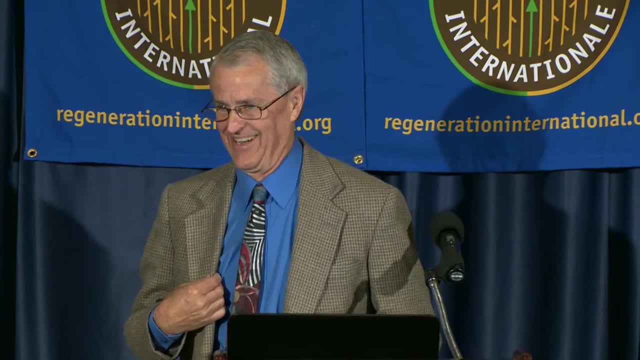 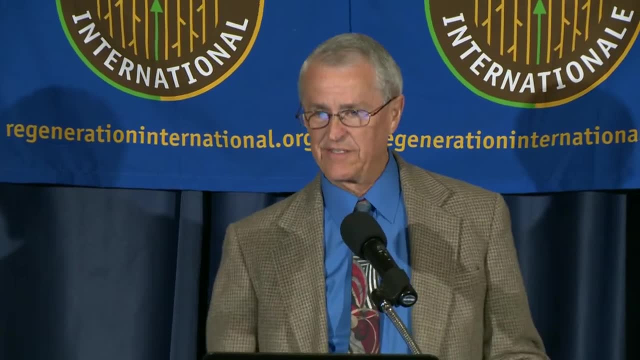 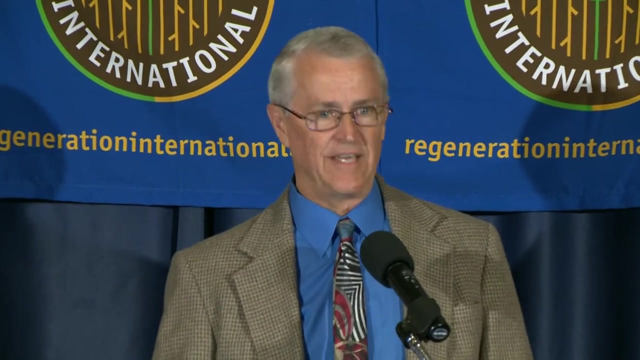 Thank you, Thank you. Have you ever had that experience in corporate where the boss comes in and says we're going to do this, this, this and this, and all your coworkers are saying yes, yes, we can do this, And the boss walks out and the blood runs out of their face and they 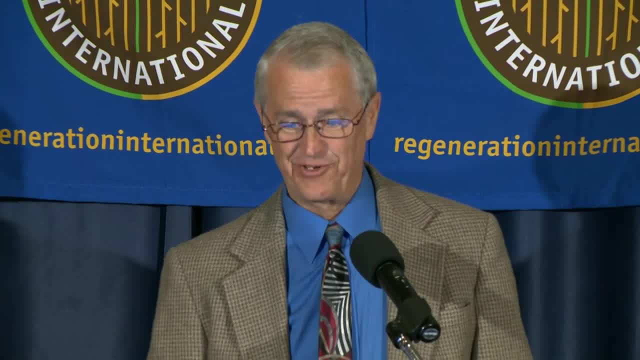 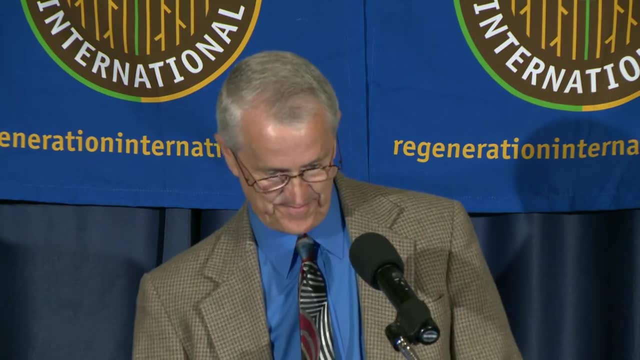 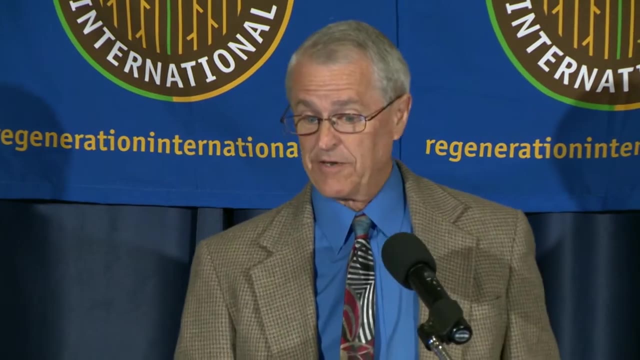 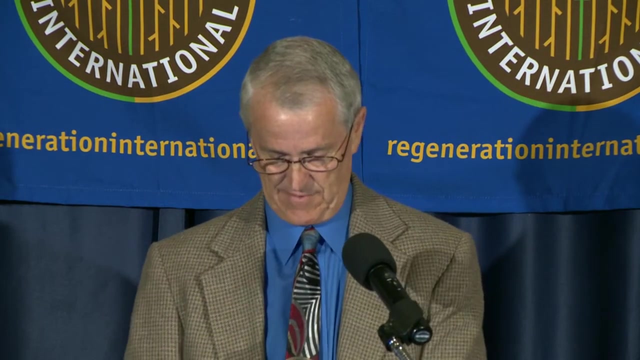 say: how are we going to do this? Well, I hope to give you somewhat of a path to the life forward on this. From a molecular biology perspective, life is turning out to be much more complex than we could have ever been able to imagine. For instance, here we have hemoglobin. It's a 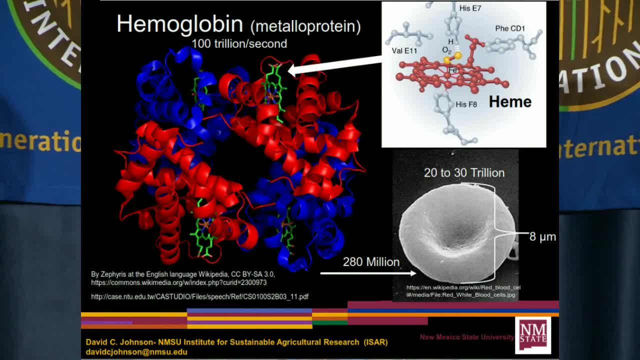 metalloprotein. It facilitates binding and release of oxygen through combining organic protein structures with inorganic metal like oxygen, Okay, iron in this particular case with a heme structure. This particular combination gives you about a 70 times increase in your blood oxygen carrying. 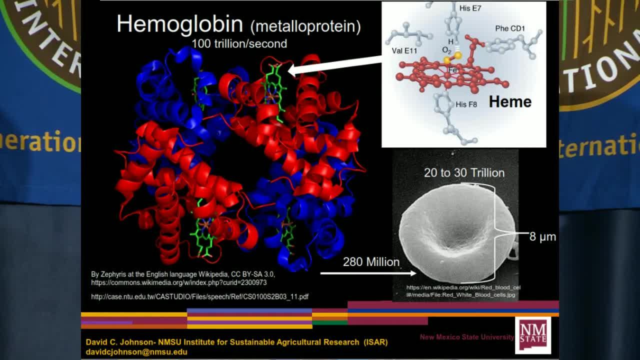 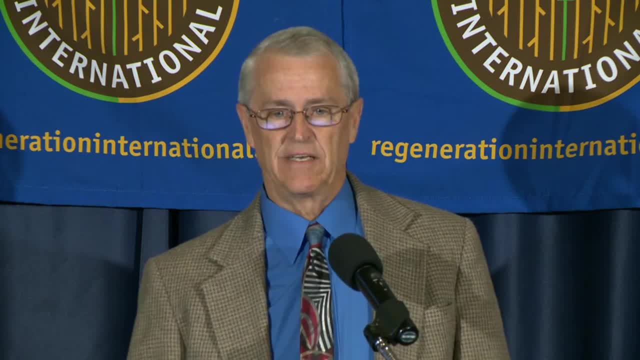 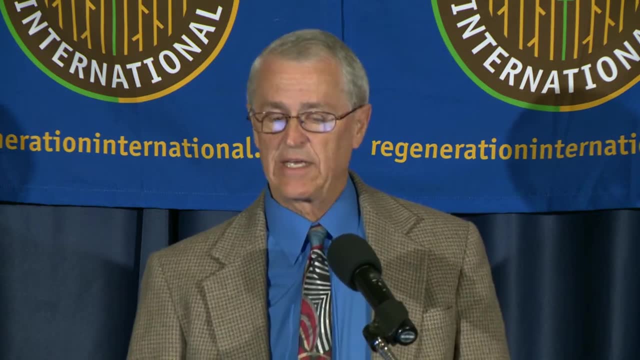 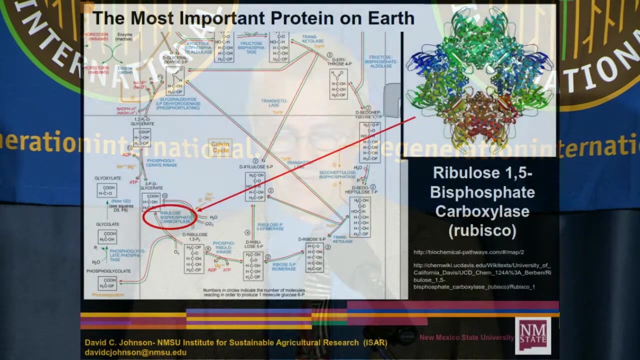 capacity and it operates, as you can see, on a time frame that we have difficulty conceptualizing, with 100 trillion of these hemoglobin molecules being made every second in our body. So life is an interplay between organic and inorganic constituents. Another protein structure, possibly the most important on Earth, is what makes life possible. 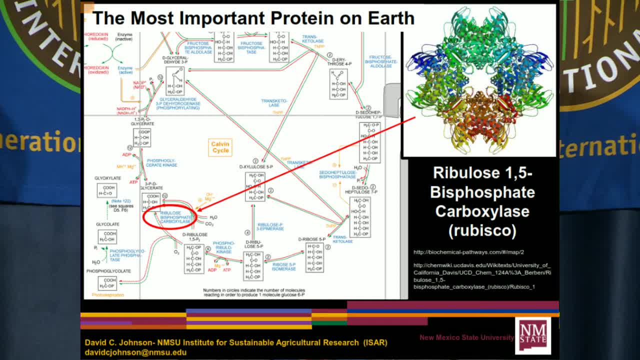 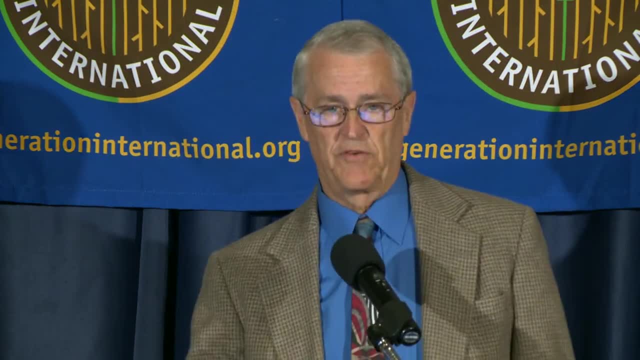 on this planet. It's made indelible changes and it's made at a rate of about one ton per second. Every person on the planet is supported by about 100 pounds of Rubisco. For the last century, we have approached agriculture from a particular perspective. 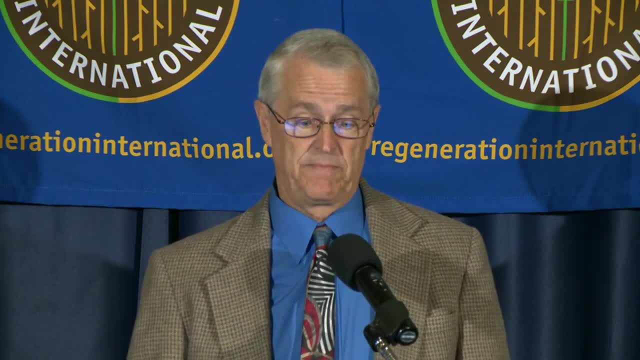 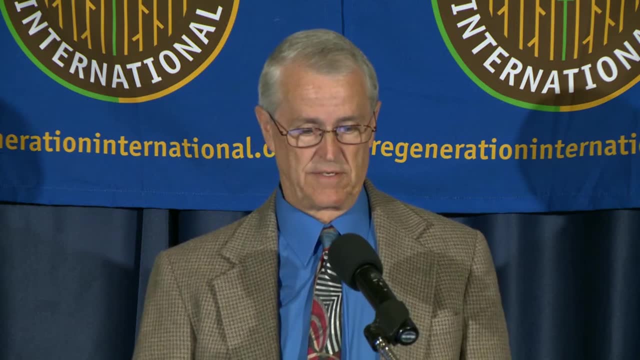 Predominantly inorganic perspective. It may be time for us to better explore the organic portion and begin considering using biology to help solve some of our problems. The question is with regards to carbon sequestration: can microbes influence the rate of carbon? 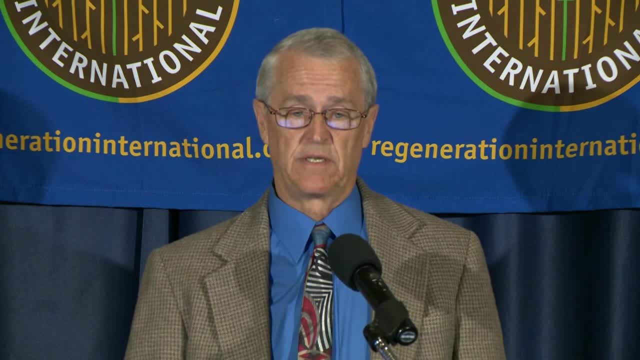 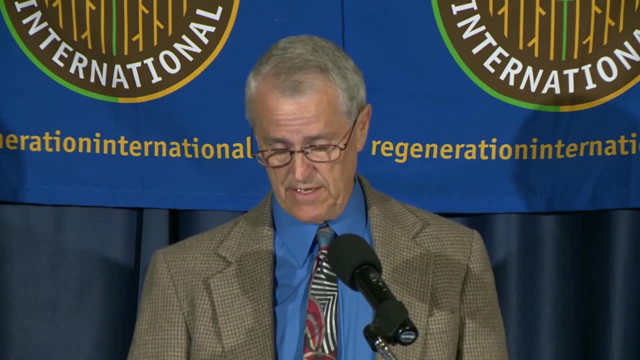 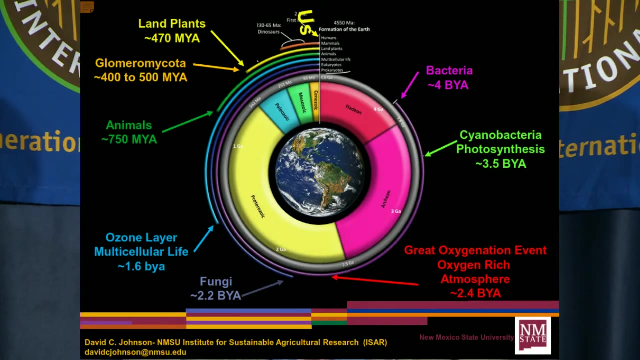 capture, input and storage into the soils of our ecosystems? And can microbes also reduce the respiration rate of CO2 from soils so that our carbon in is greater than our carbon out? Microbes have been integrated into our ecosystem. They've been integral in shaping our Earth for the last four billion years. 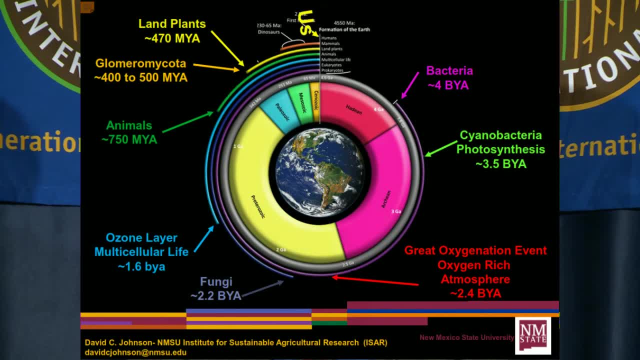 We are a living planet. That's what makes our planet different from all the others. As you can see, about 3.5 billion years ago, nature developed the possibility to store energy through photosynthesis, to capture and store it. That led to the great oxygenation event, which poisoned the atmosphere for the anaerobes. 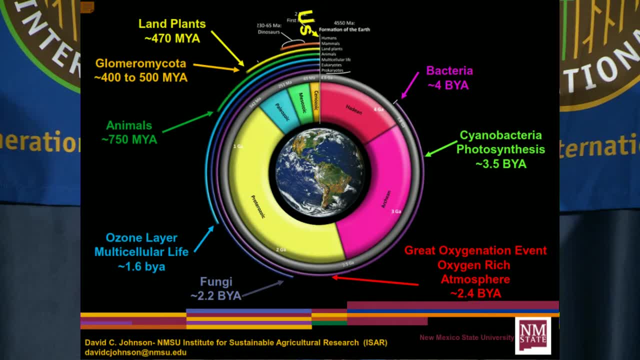 but it led way for fungi to develop, led way for the ozone layer, Animal life evolved And, as you can see, about the same time land plants came along. the Glomerulocicata, this is a mycorrhizal fungi that associates with roots of plants to help them get the nutrients. 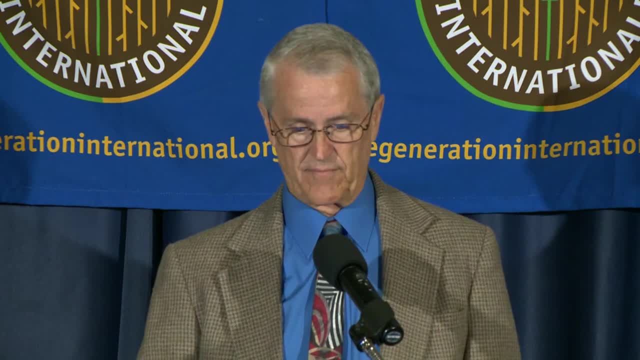 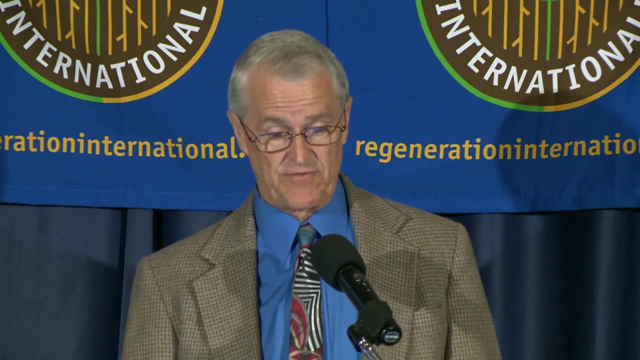 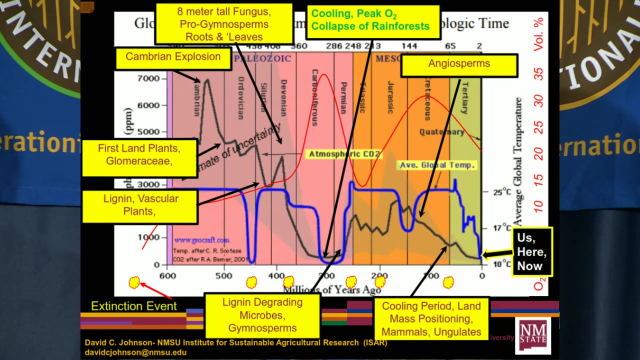 they need. They came along about the same time. It's also interesting to note the influence of microbes and other life forms on carbon capture abilities and atmospheric CO2.. The black line on the area is the atmospheric CO2.. The red line is oxygen and the blue is Earth's temperature. We're about there right now. You can see back in the Cambrian explosion. when organisms developed the ability to use calcium carbonate in their shells, you had an explosion of life, So you had a reduction of CO2 in the atmosphere. First land plants came along about 500 million years ago. Same time as Glomeraceae, They started reducing it more And about. in the Silurian, about 408 million years ago, lignin was developed- vascular plants, You can see you have another decrease And then in the Devonian you had about eight meter tall fungus progymnosperms. 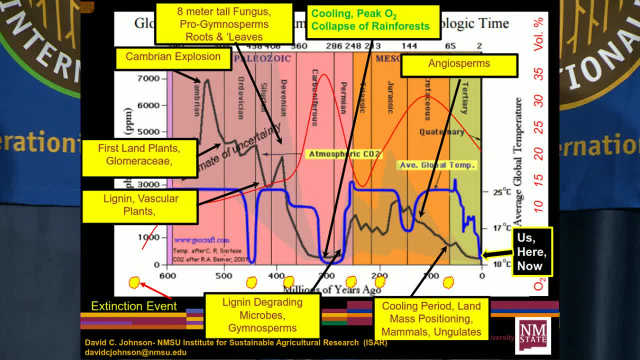 Again you got another decrease And then you had a cooling period. The carboniferous period was a quite long period. You had a cooling period. It was a quite productive period for all the carbon that was put in our soils. That's where we get our coal, a lot of our oil. 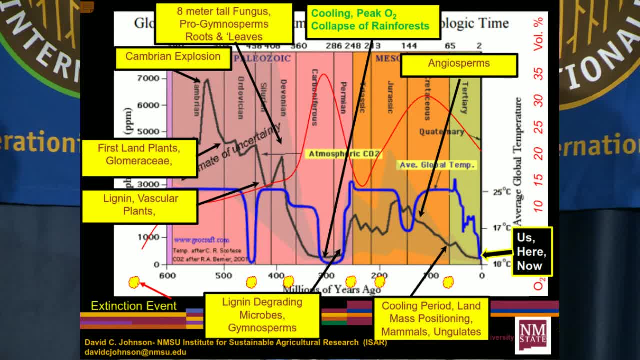 But then along came lignin, degrading microbes. You start to see an increase in the soil carbon, I mean in atmospheric carbon. Angiosperms came along about 100 million years ago. You can see another decreased start And then you had another cooling period and this is when the land mass positioning and 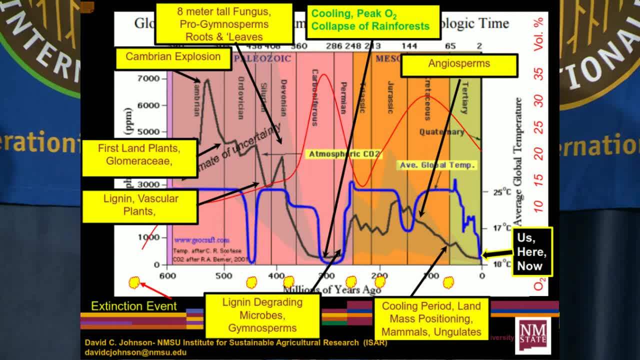 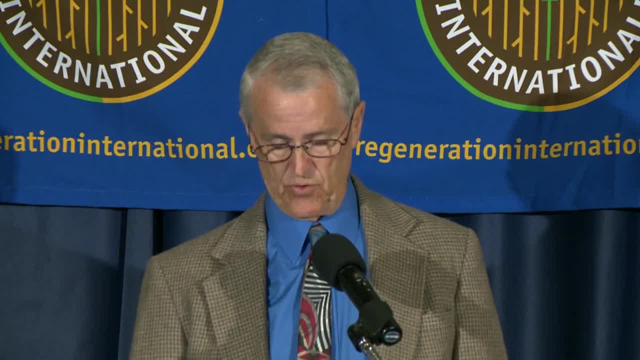 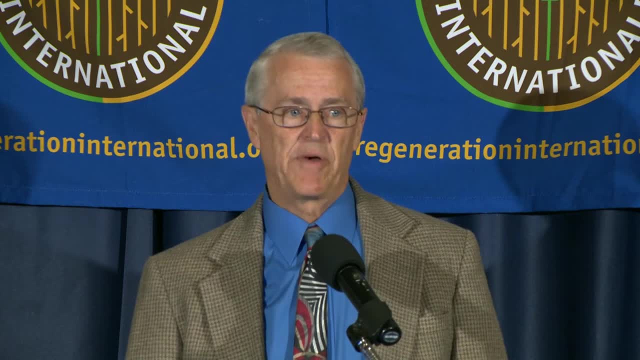 mammals, You know ungulates grazing on grass. they start to reduce the atmospheric CO2.. So how intimate is the relationship between microbes and other organisms? In humans we're outnumbered: 10 to 1.. When you consider the number of genes, we have about 30,000 genes. 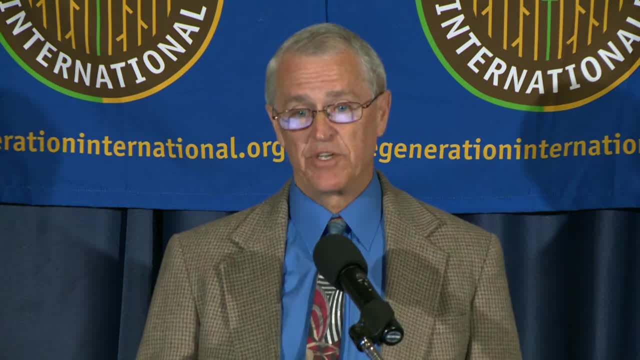 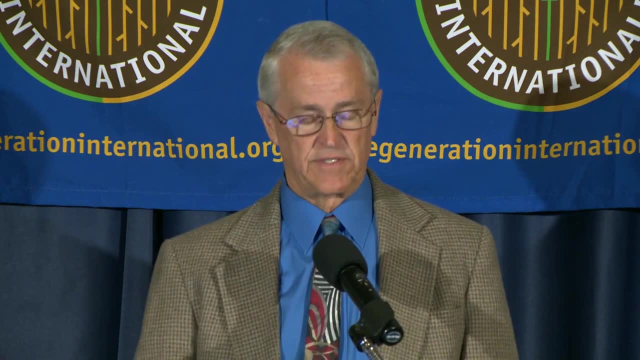 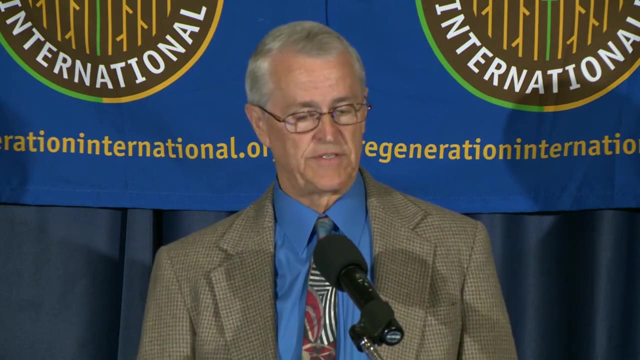 Our microbial complement has 8 million, So we're numbered 250 to 1 in this arena. So life forms on this earth have evolved as super organisms. So what do microbes do for us? They help digest our food. they generate nutrients for us, they synthesize vitamins, break down. 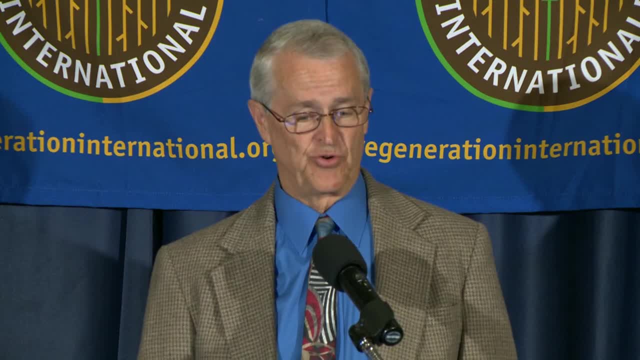 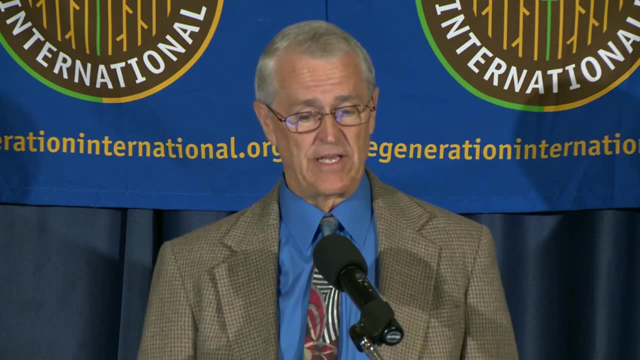 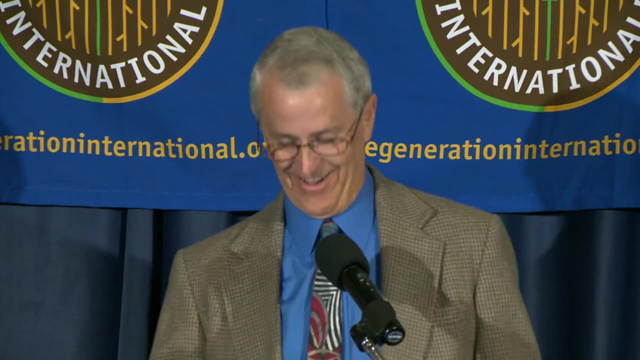 xenobiotics. detoxify carcinogens, promote cell renewal, activate and support your immune system. control our appetites and cravings, turn on and off our genes in our body that regulate brain development, anxiety, depression and emotional behavior. You're working on me right now. They prevent asthma and skin diseases in infants. They prevent cancer. They stimulate alcoholics, alter immune system development, promoting or avoiding allergic disorders in later life. If disturbed, these functions can be compromised. Crohn's disease was once very rare It's over the last 10 years. it's increased 10-fold in England in 16- to 29-year-olds. Now, instead of prescribing more antibiotics and intestinal resections, doctors are starting to use fecal transplants to cure Crohn's 1. But in some cases the cure is within 24 hours. So plants are no different from us. They also are outnumbered by their microbial counterpart. 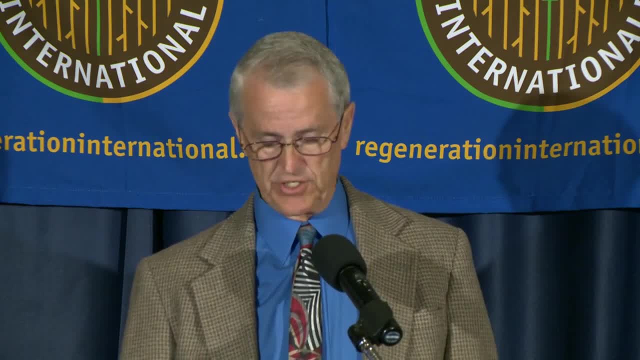 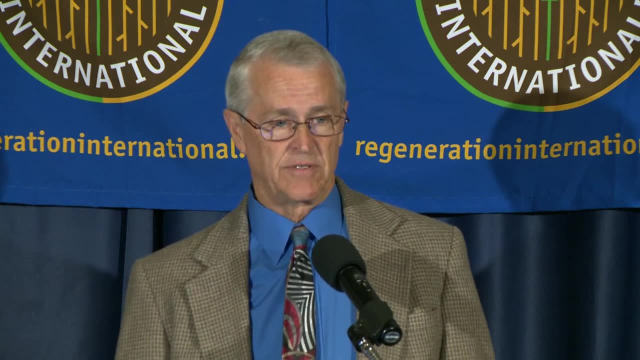 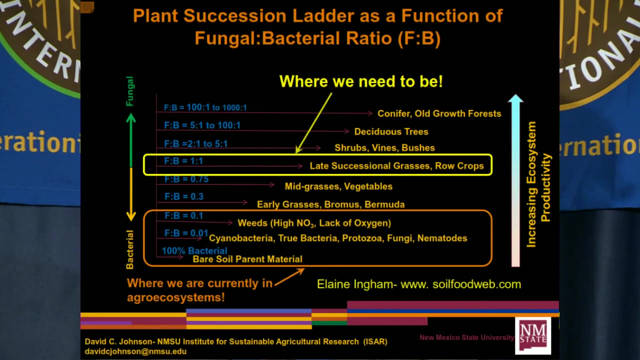 and depend on them for nutrient acquisition, pathogen protection and gene regulation. So if we can fix human micro-omes, can we do this in agriculture and rangeland soils? Can it be this easy As you shift from bacterial dominance to fungal dominance in the soil? 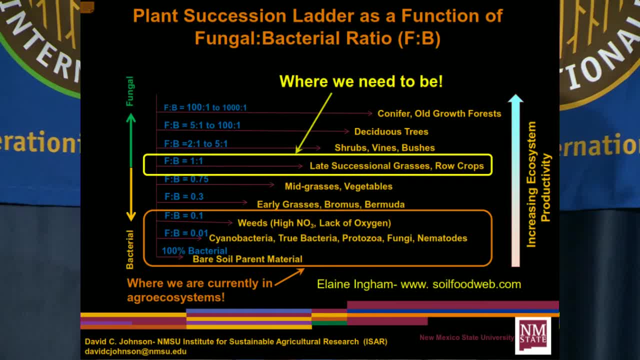 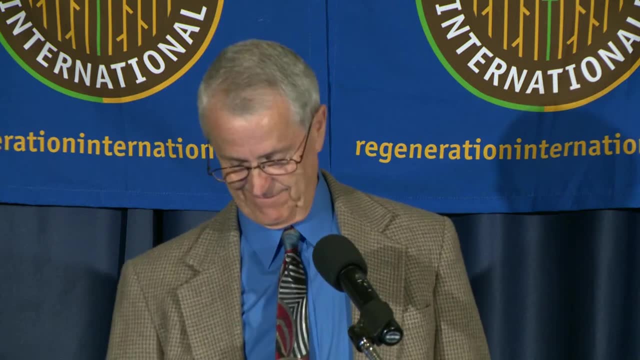 we see fertility and ecosystem productivity both increase, along with the type of plant that grows optimally under those conditions. Note two things. Currently our agricultural system is about .2 in the fungal to bacterial ratio. What we grow best are weeds. We need to be up about one to one. 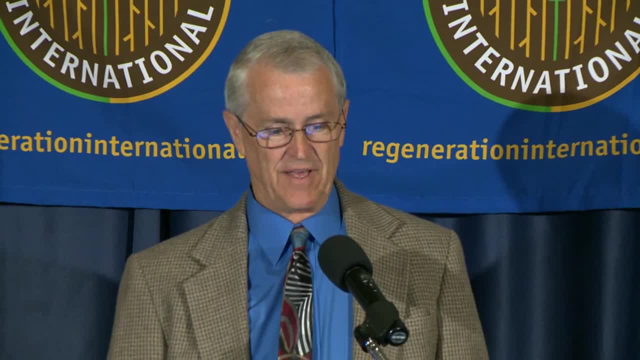 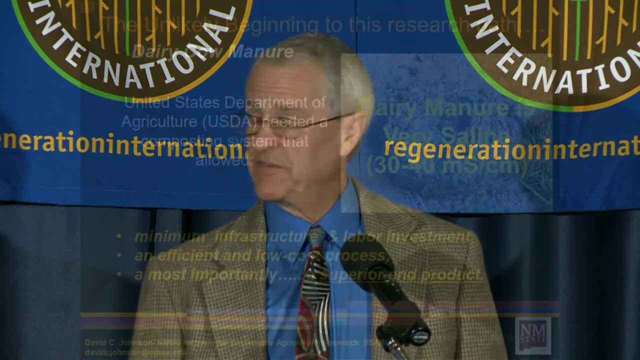 to be able to grow plants that we like to eat. The unlikely beginning to this research path was a project with USDA, And I received this the second day I got to work And you can imagine my excitement on the project that my boss gave me. 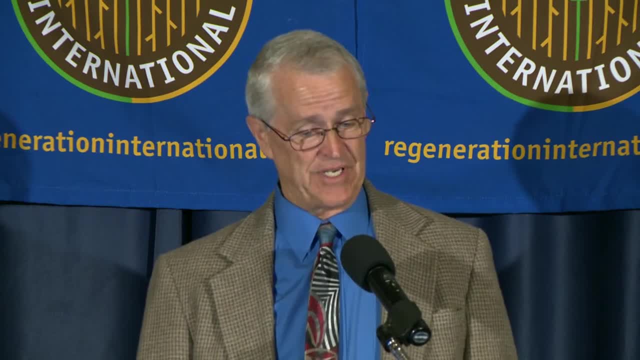 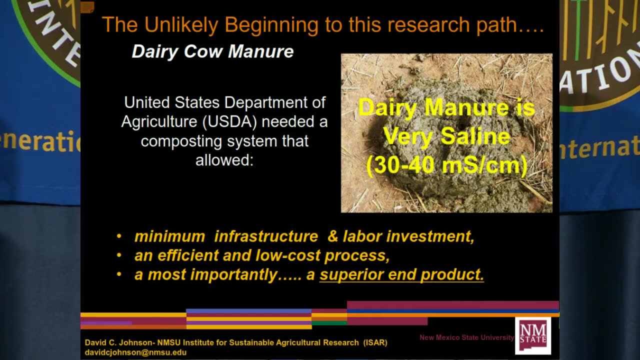 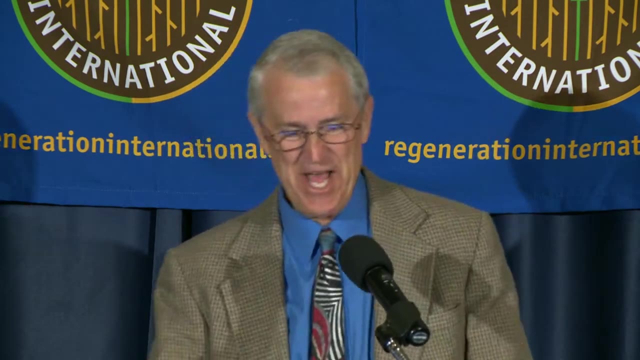 He did me a big favor. So USDA needed a system that had minimum infrastructure and labor investment, an efficient and low-cost process and, most importantly, a superior end product. Problem was Dairy manure is very saline. It's about 30 to 40 millisiemens. 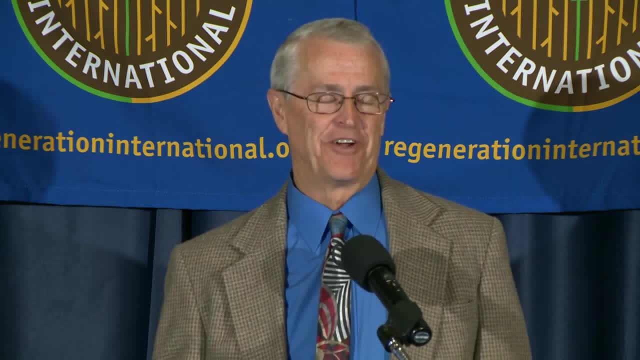 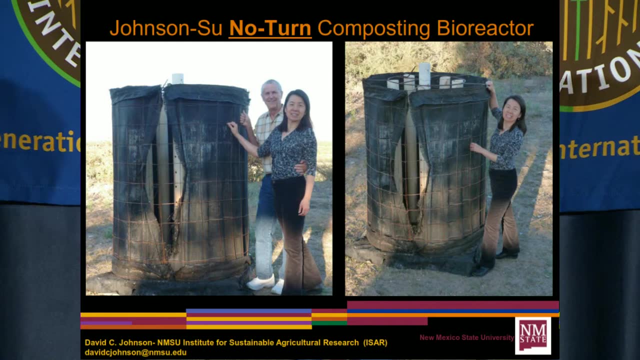 So my wife got tired of me coming in with manure all over my clothes from turning the piles, So she helped me develop a no-turn composting bioreactor. And that led to the rest of my research. Because what that technology did, it gave us a composting process that reduced water by a factor of six times, reduced composting time by 66%. It resulted in a low salinity compost, which you know in our area it usually gets worse when they do the windrow composting. 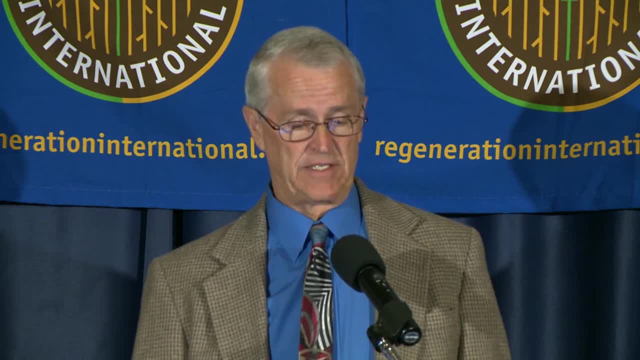 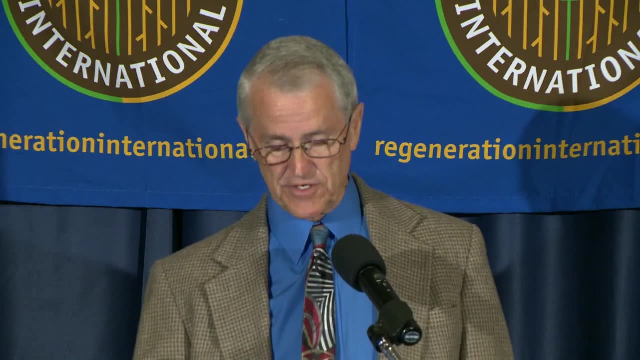 It's amenable to incorporation of vermicomposting after the thermophilic phase. But, most importantly, it produced a high-quality, nutrient-rich, fungal-dominated compost, And this fungal-dominated compost is what allowed me to continue my research in this area. 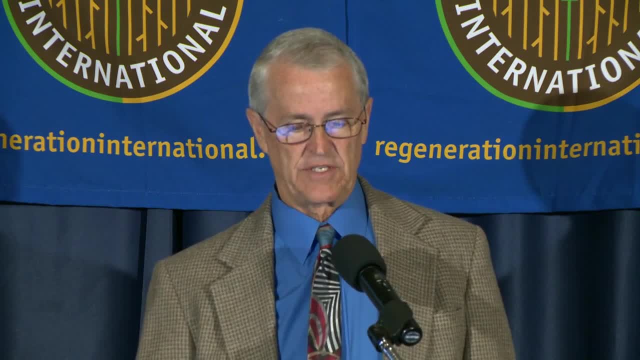 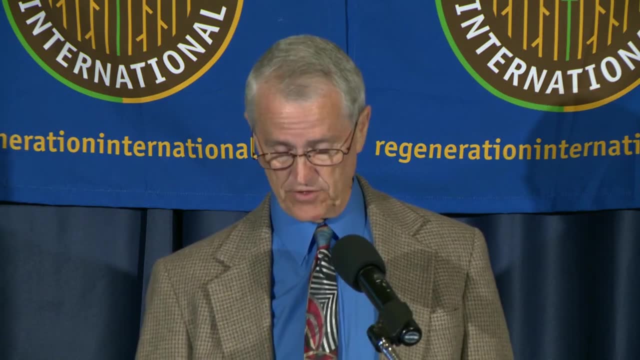 So we did a test with eight other composts in that area And we did basically the standard composting. We did the standard soil test along with the biological assay to assess the fungal-bacterial ratio. As you can see: nitrogen, phosphorus and potassium. 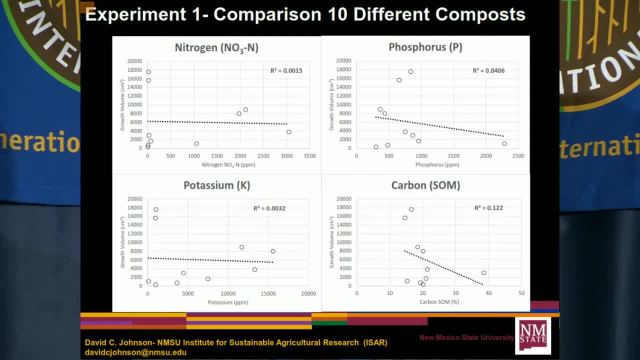 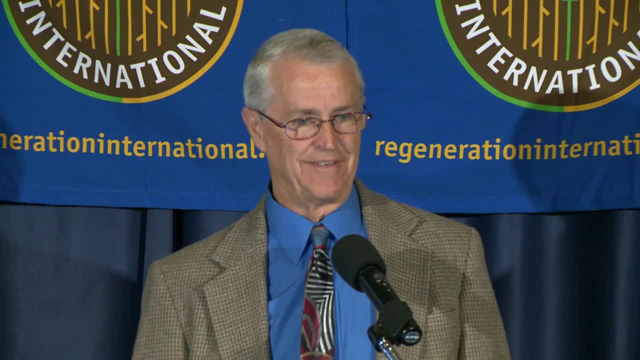 did not correlate well to plant growth And, to my surprise, neither did carbon This kind of. I was expecting carbon to be at least one of the correlating factors. Fungal-bacterial ratio. however, we had our R squared of 0.87.. 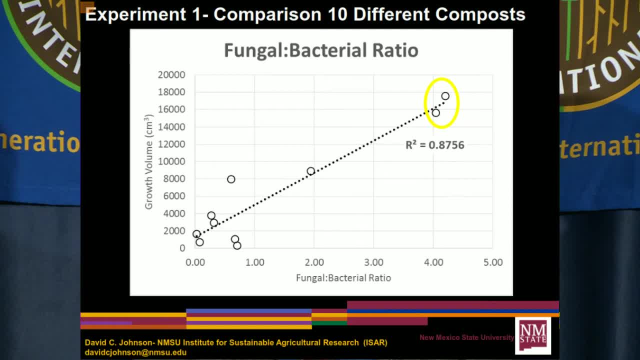 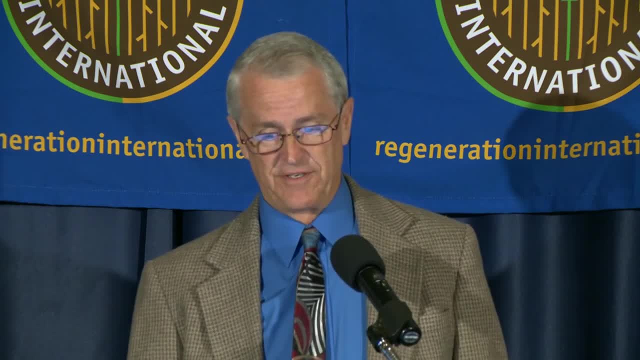 And the compost that we produced, which are these top two, produced twice the plant growth of any other compost. So a second experiment was developed where we could look at increasing soil carbon percent, And the soil mixtures were made from an arroyo sand. and this compost that we produced in this reactor. Experiment two demonstrated that 70% of the total carbon assimilated by the plant was returned to the soil. From a survival standpoint, it seems odd that a plant would develop that much energy to the soil. 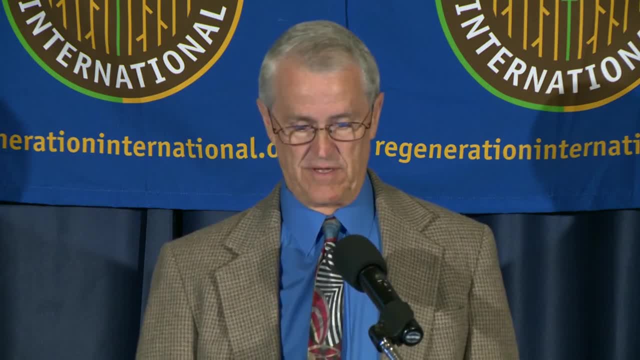 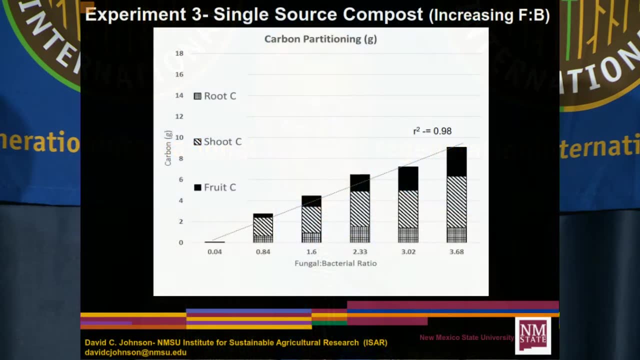 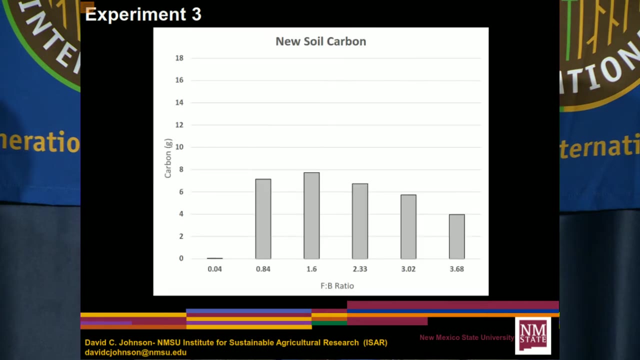 unless there was something important going on there. A third experiment looking at influence of fungal-bacterial ratio on carbon partitioning. Here you can see the flow of carbon into the plant biomass- It's pretty much linear. And here you can see the flow of new soil carbon. 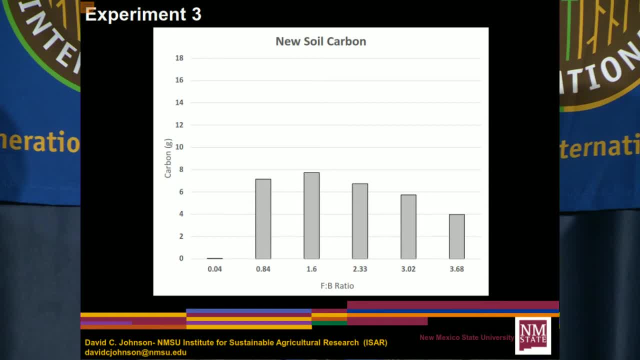 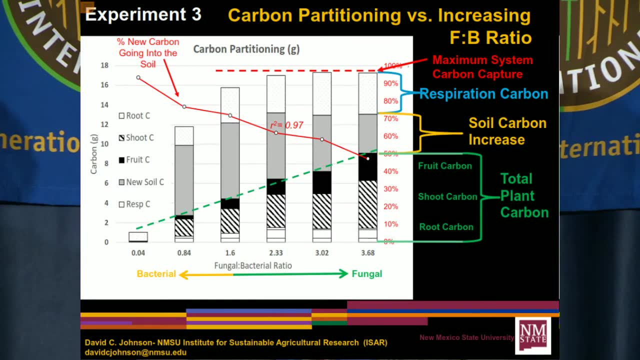 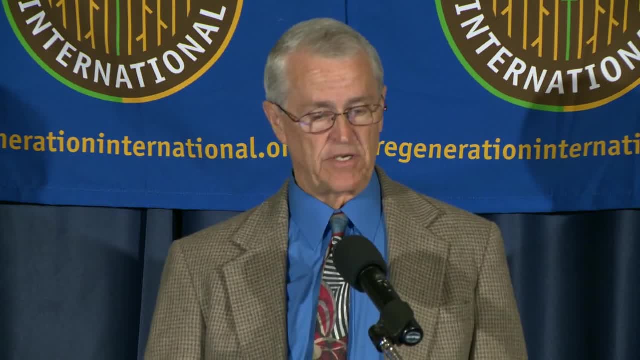 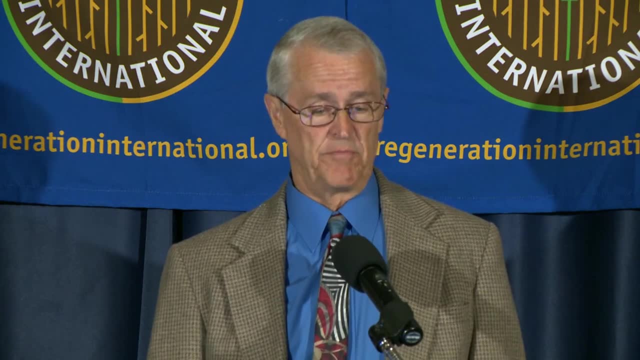 how will a biologically enhanced soil, how will an agglutinous agricultural management approach work in the field for increasing carbon? G Beam Implementation uses inoculation of soils with its Fungal-dominant compost. only 4 to 500 pounds per acre. 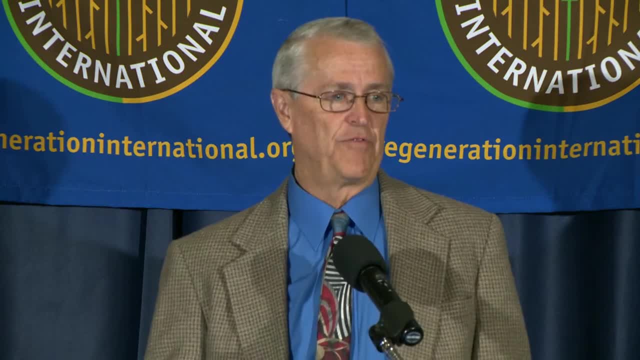 You can spread it, spray it, irrigate it, coat it, inject it. you can spread it, spray it, irrigate it, coat it, inject it. however you want to do it, You generate. basically, it's like a dough. 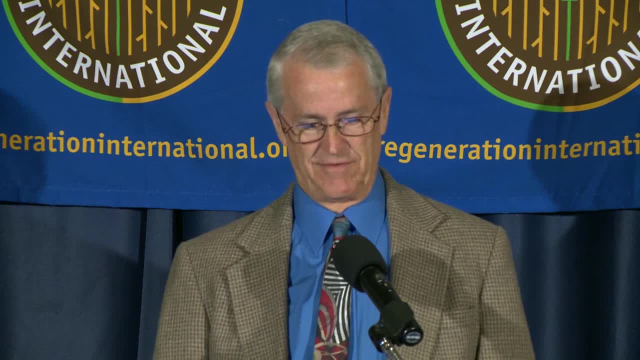 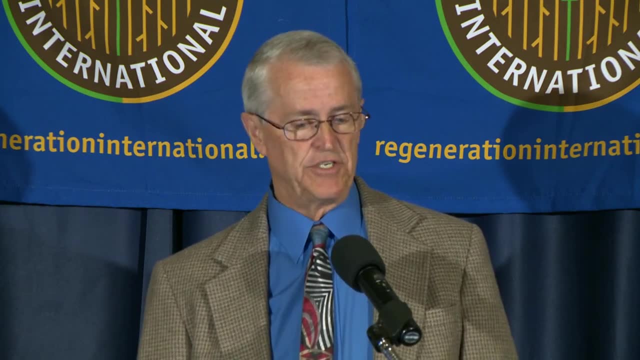 You're adding a yeast and that kicks the whole thing off. Plant Cover Crops designed for building soil nitrogen Never bear fallow. Harvest as much energy you can on the soil area you have, as soil carbon is the key to microbial population increases. 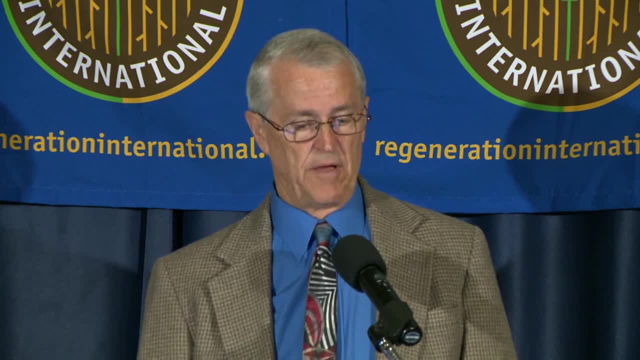 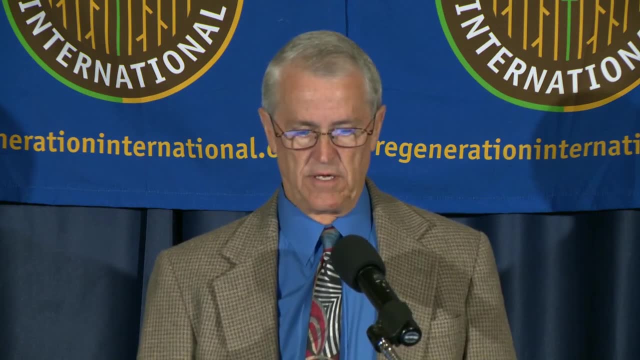 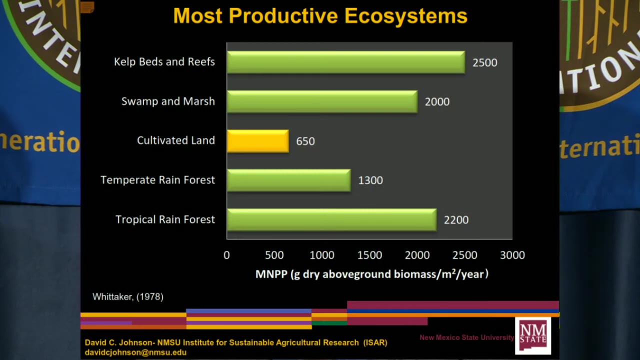 mutualisms and the synergy development Manage for the microbes. Low to no fertilizer applications, No herbicides, No pesticides. So in terrestrial ecosystems you can see swamp and marsh, and the tropical rainforest produce about 200 to 2,200 grams of dry above ground biomass. 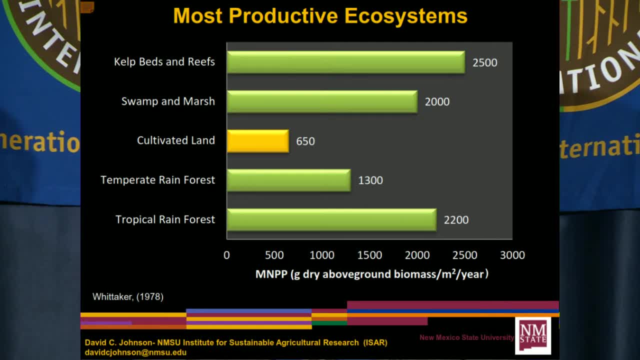 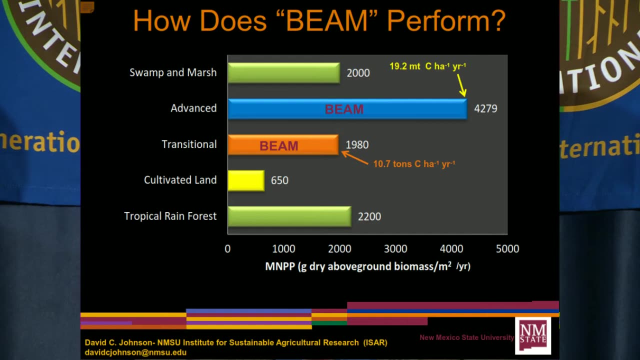 per square meter per year. You can see we do not do too well in cultivated land, Even though we can water it. we can weed it and we can put fertilizer on it. So in my bean trials I've averaged 1,980 grams. 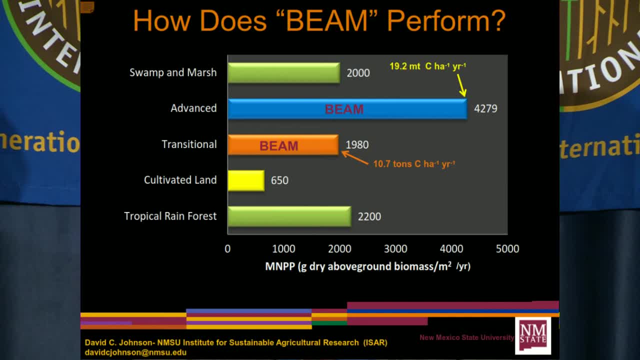 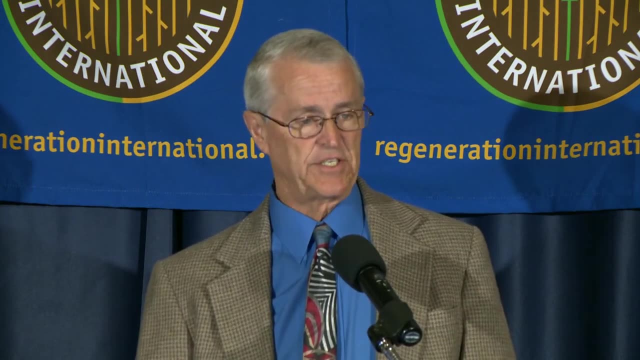 of dry above ground biomass per square meter a year. So I'm up there, close with the most productive ecosystems on Earth. In my advanced bean I've produced 4,279 grams, That's 1,980 grams of biomass. So those will lead in my transitional bean. 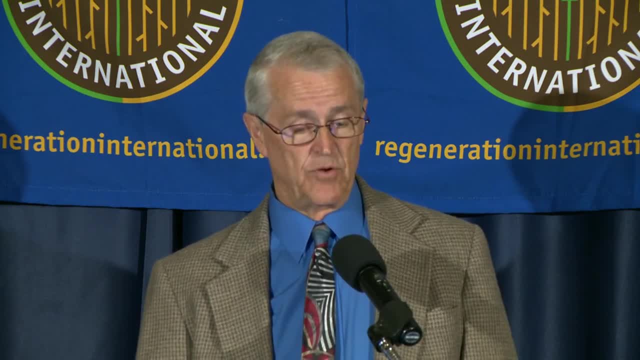 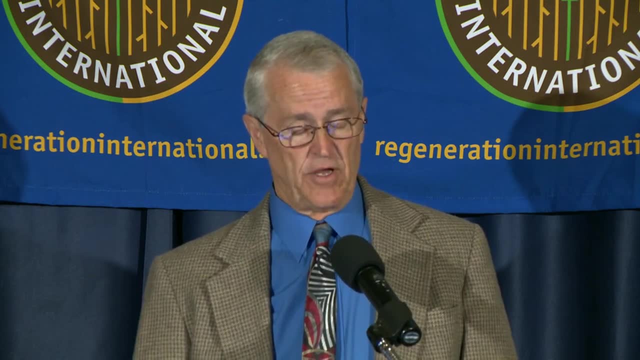 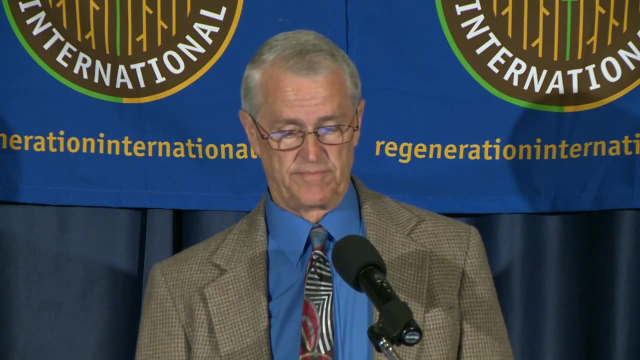 it'll lead to 10.7 tons carbon per hectare per year, which is about 37 tons of CO2 per hectare per year, And, of course, in the advanced potentially we can see 19.2 metric tons of carbon per hectare per year. 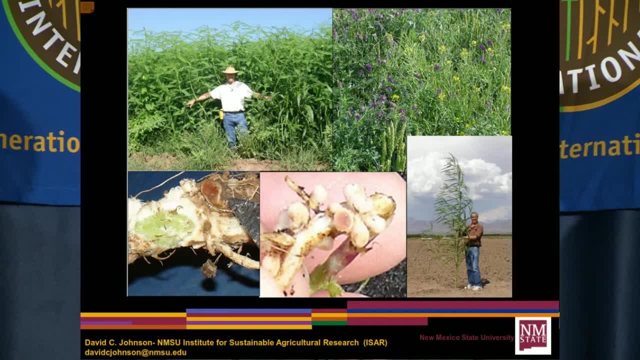 These are some samples of the cover crops we used in this research. Suspania: it's a legume. It associates also with ectorhizal fungi And in the first season we grew it. it only grew about four feet. 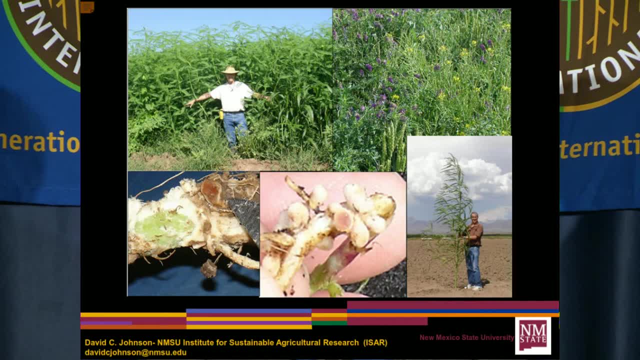 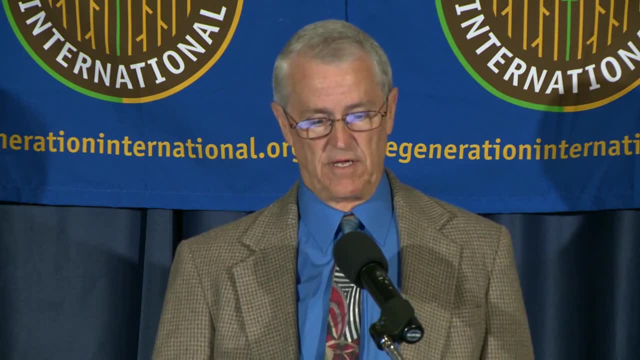 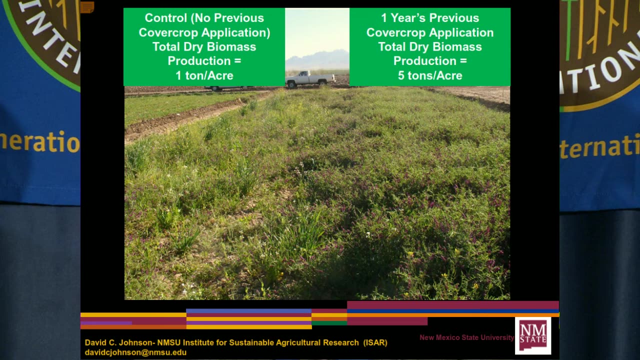 The second season, six feet And by the third season it was 12 feet tall. We were improving the soil every time that we planted, plus all the other processes that we did as far as inoculation. This is a comparison of one year's application of beam. 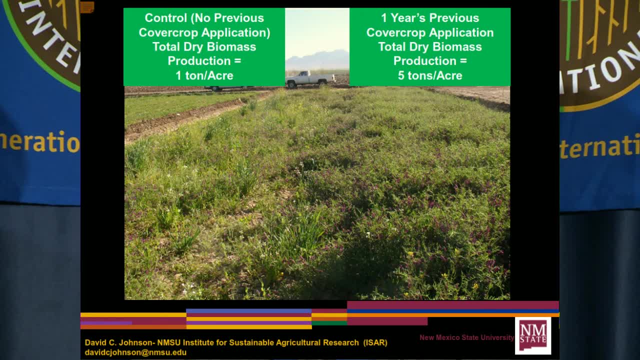 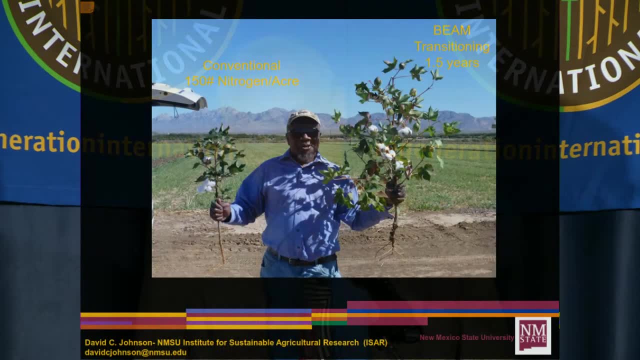 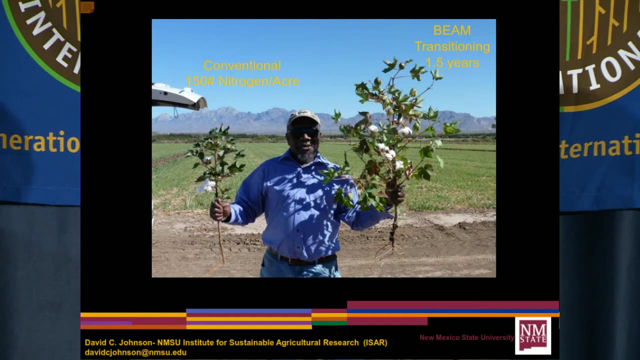 with a side-by-side control with no previous cover crop yielded a five times increase in biomass over one year. This is a scientist from Los Alamos, James Barefield. We also planted some cotton in these fields to compare conventional approaches to beam. 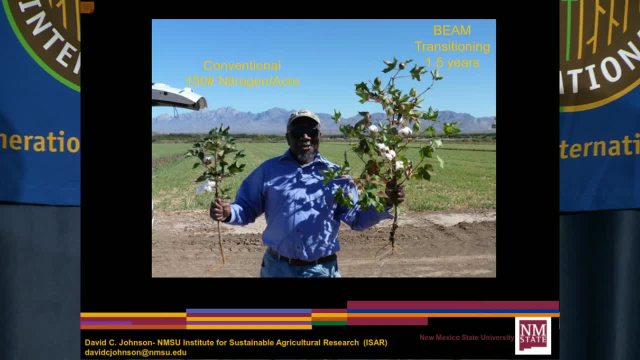 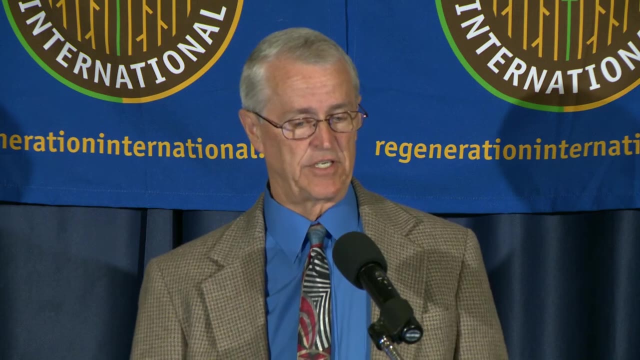 You can see on your left James is right. the conventional is 150 pounds of nitrogen per acre. On the right is the beam transitioning. after 1.5 years We doubled the productive capacity of that Soil, just with biology. Commodity crop wise, we looked at cotton and chili production. 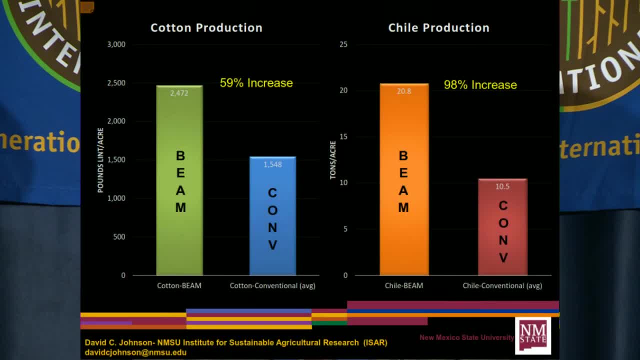 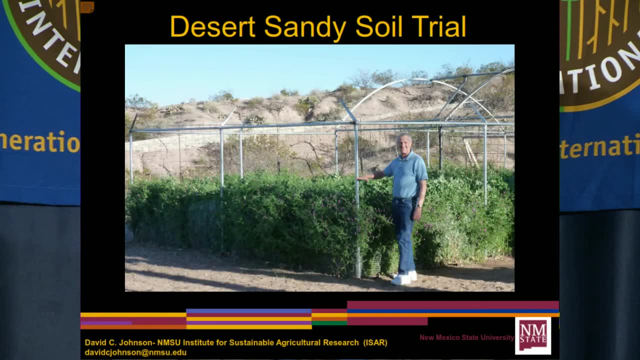 In cotton we had a 59% increase. In chili production, we had a 98% increase just using beam. A fourth growing period on this. this is a desert sandy soil trial. On this one I've come in, I've inoculated. 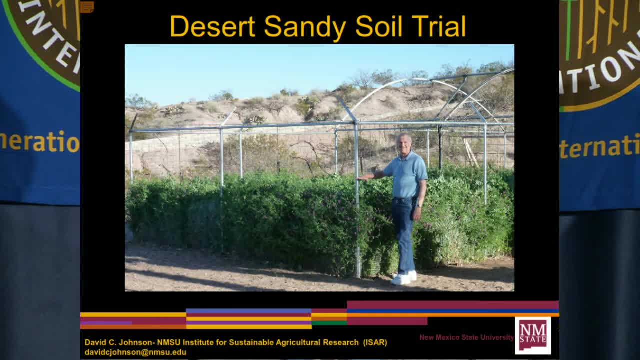 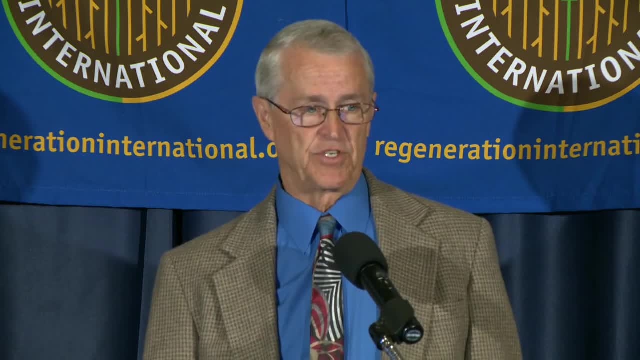 and I've grown a crop, I've cut it, hauled it off and then planted another crop. This is our fourth growing period on this And we yielded 60%. We yielded 1,604 grams of dry biomass per square meter. 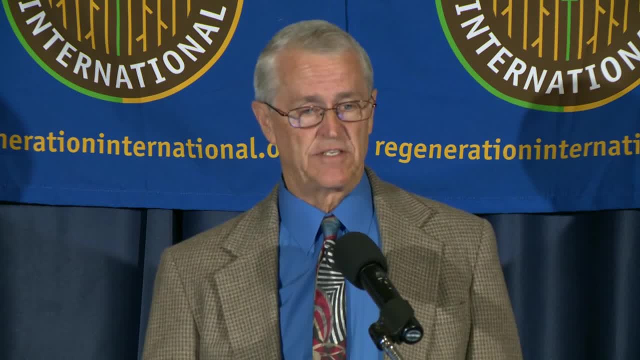 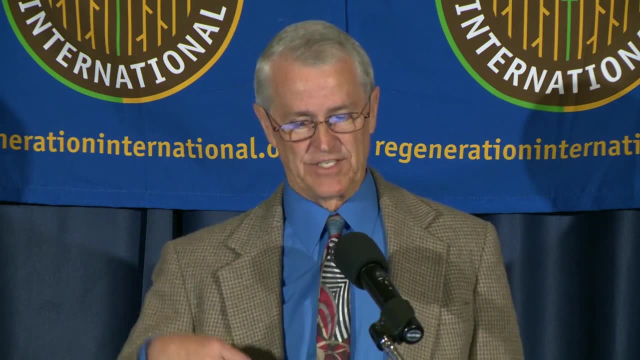 on this particular one. To give you an idea, that's about 6.5 tons of dry biomass. In our area that is a full summer's production on alfalfa. So this was in a winter cover crop So I still had the rest of the growing season. 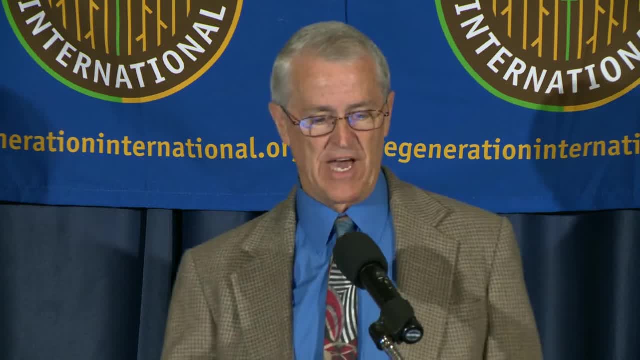 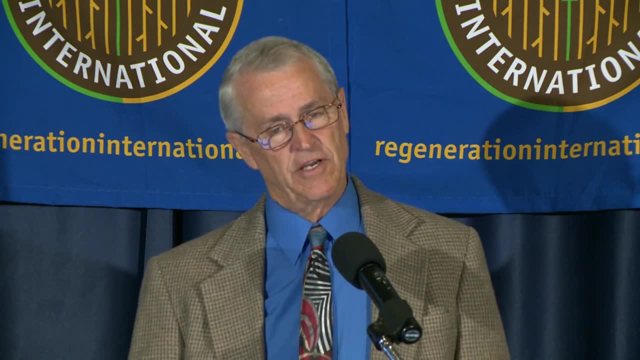 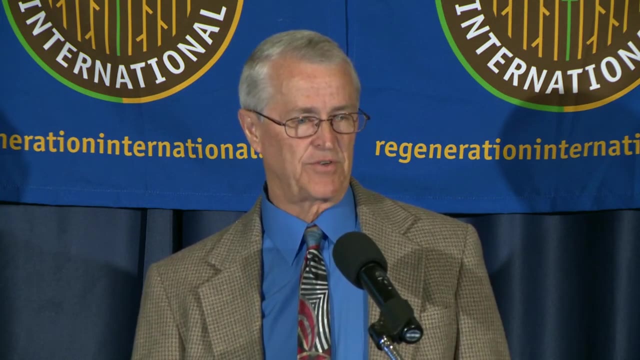 to accomplish more. So how does a biologically enhanced agriculture management or beam approach work for decreasing carbon out? And here's where we vary a little bit, depending on what scientists are seeing, At least the ones that are developing the models for the carbon flow out of the soils. they usually say that the more carbon you have in the soils, the more carbon you can respire And, as you can see, yes, there was an increase in respiration in this, But when you consider that, I have a 20 times increase. 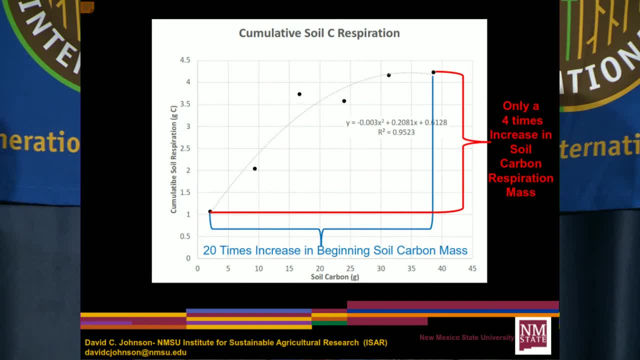 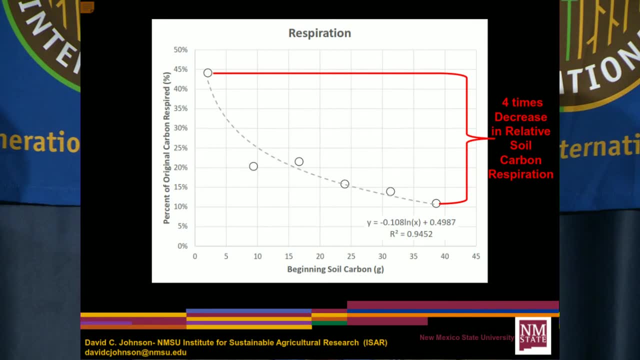 in beginning soil carbon mass and only a four times increase in soil carbon respiration. So we've been able to reduce the soil carbon respiration by four times. In the low fertility we had 44% of the beginning carbon respire. 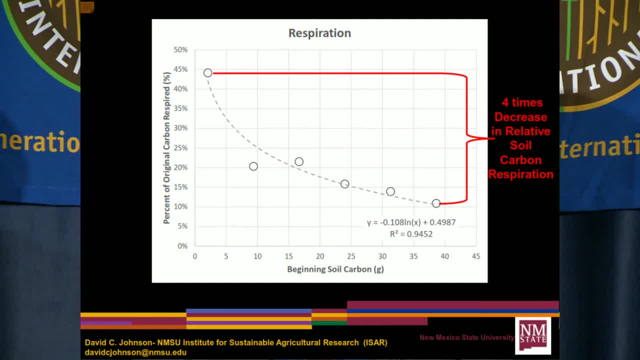 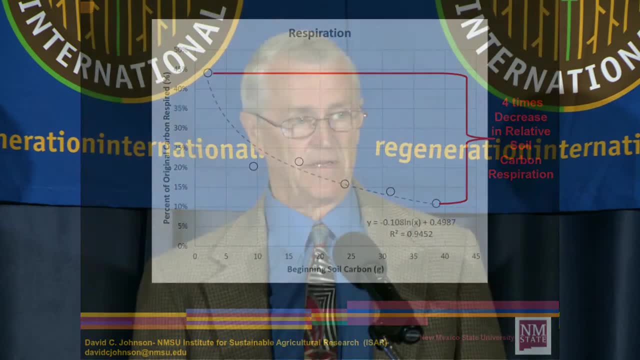 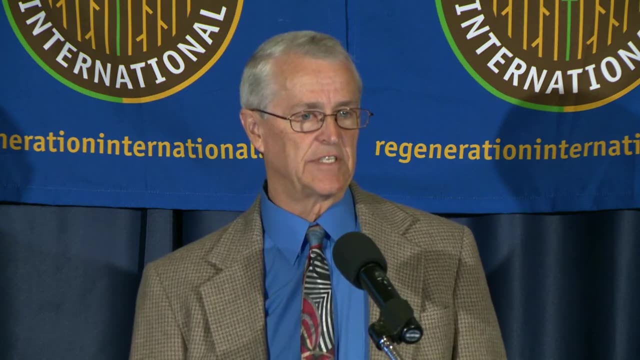 Where in a more fertile or the fungal, higher fungal ratio, we had a four times, we only had 11% of that carbon respire. So it's again it's biology that makes this happen And it's increasing the carbon use efficiency. 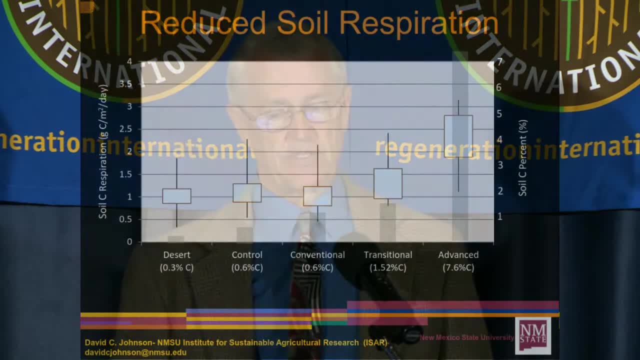 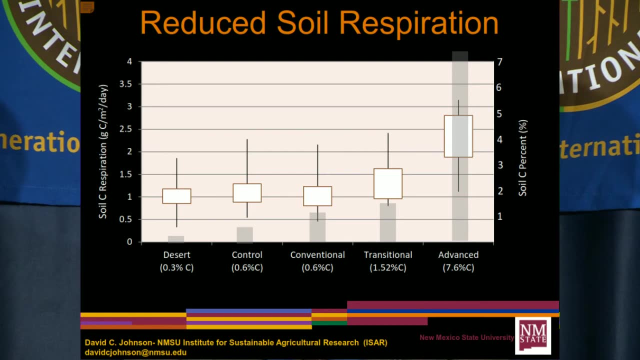 of this system underground. This is a one-year study of samples comparing respiration in five different soils, from a desert soil to an advanced beam soil. You can see I have a seven times increase in the soil carbon, yet we only have a doubling of respiration. 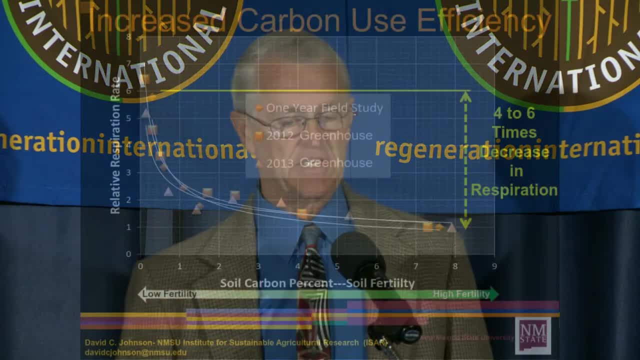 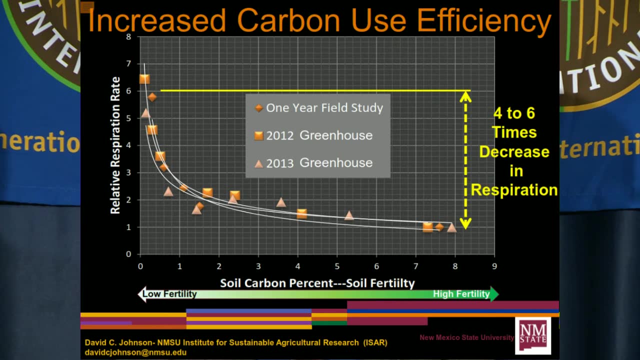 This is all of them put together. You can see there's a pretty good agreement on how this works: that as you improve soil fertility, as you improve the fungal to bacterial ratio and start to work on the biology in soil, you get less respiration. 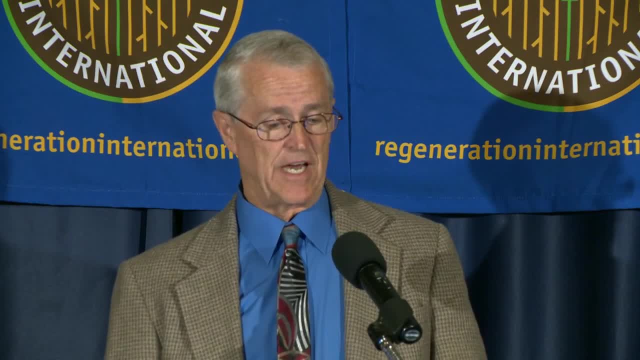 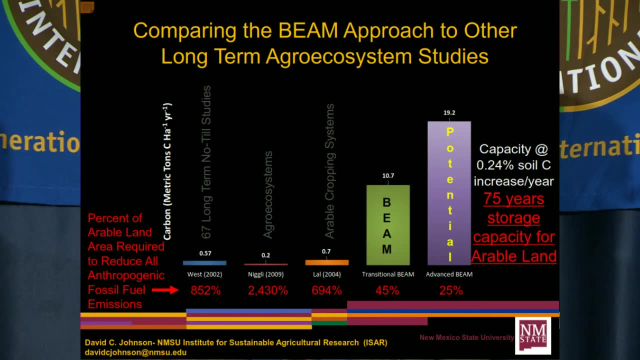 So as we shift soil microbial dynamics from bacterial to fungal dominance, we observe increasing carbon in with decreasing carbon out. Comparing beam to other long-term approaches West, with 67 long-term studies estimated we could capture 0.37 tons of carbon per hectare per year. 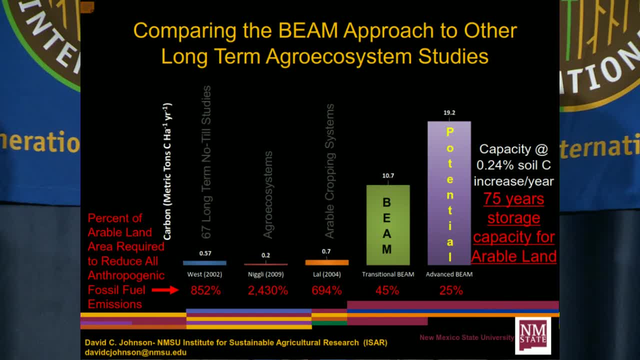 Nigley: 0.2.. Lowell, 0.7.. With beam I've done 10.7 and up to 19.2.. And the percent of arable land required to reduce all anthropogenic fossil fuel emissions. 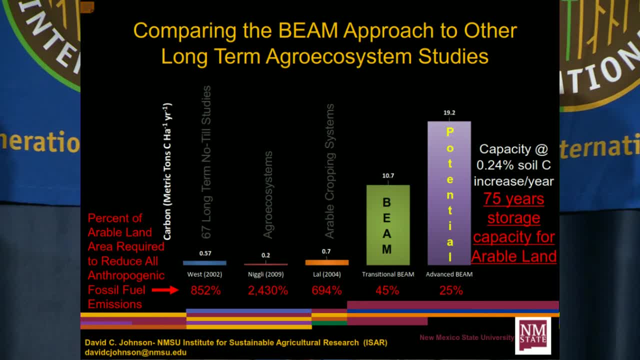 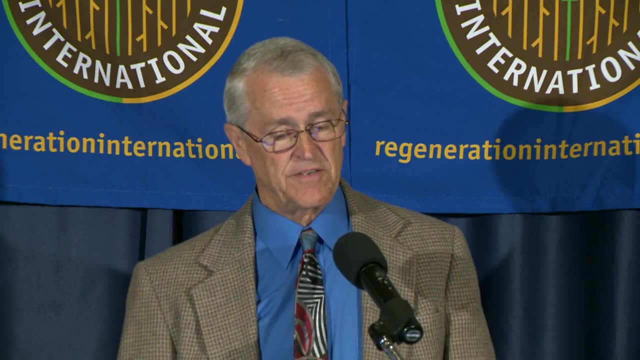 you can see it's 852% with West, 2,430% with Nigley, 694% with Lowell, 45% of the arable land with transitional beam and 25% with advanced beam. So at that, capacity of increasing the soil carbon: 0.24%. 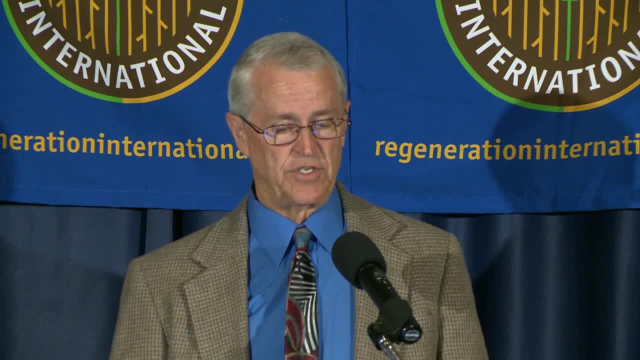 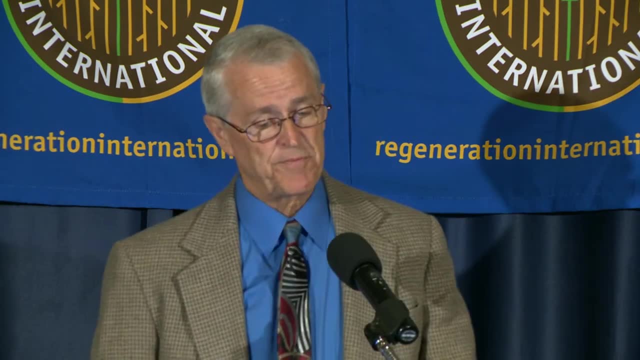 soil carbon increase per year. you have about a 75% increase, So that's a 25-year storage capacity for arable land. So we can do this By stripping carbon out of the life and the life forces it supports from our agricultural soils. 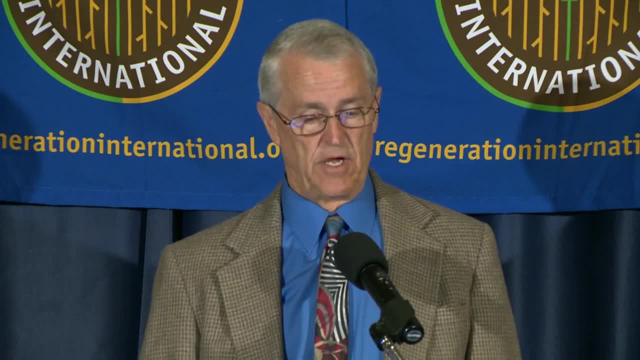 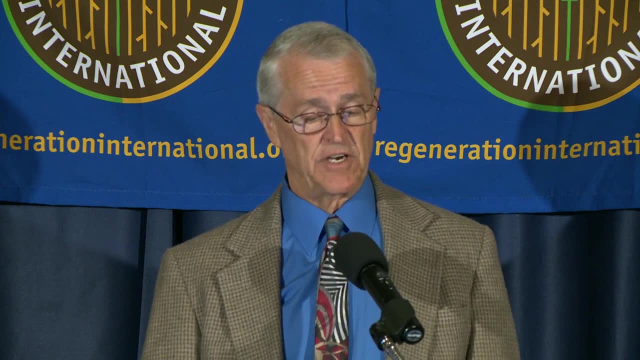 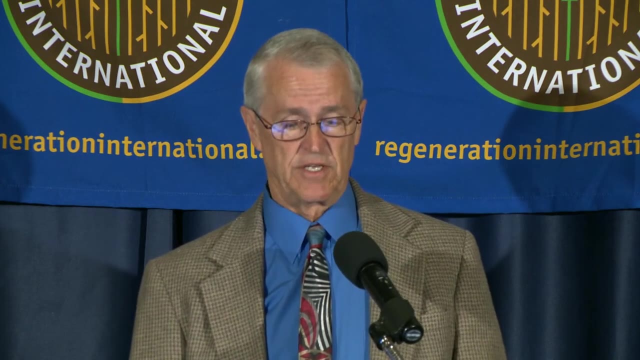 we have reduced the ability of these soils to function optimally. Restoration of soil microbiome population and its structure, along with soil carbon, promotes restoration of biological functionality of our soils. By promoting this restoration, we can begin reducing atmospheric and soil concentration. We can begin now, at any level in all ecosystems. We can reverse soil loss by restoring and rebuilding our soils. We can slow desertification. We can reduce soil salinization. We can reduce the downstream pollution from application of agrochemicals. 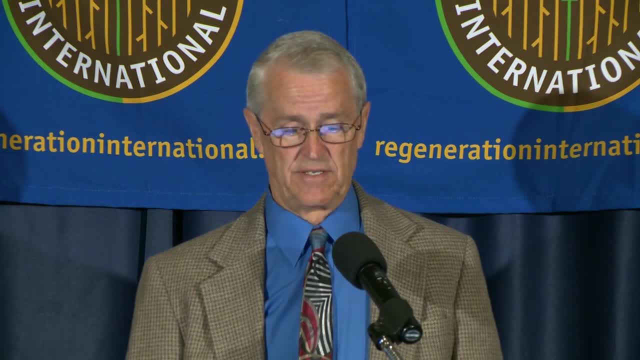 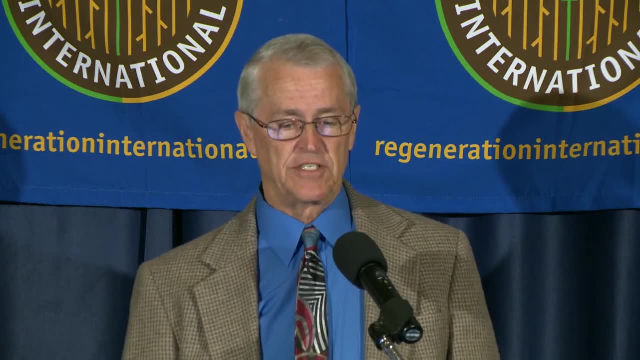 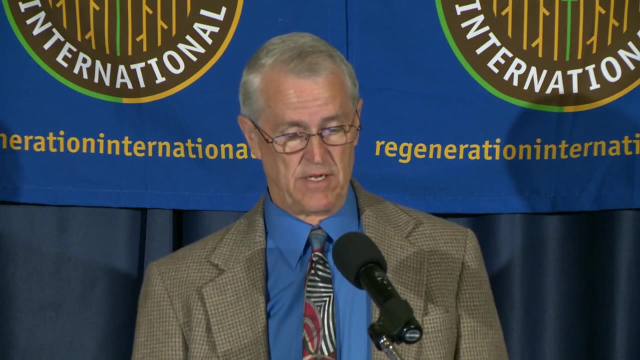 We can restore beneficial insect and pollinator populations in this, And we can begin restoring our coral reefs and our oceans also. We have a viable technology. We have a viable technology to reduce greenhouse gases, but we cannot accomplish this without a policy that supports its implementation or without the presence. of a stable and predictable market. Farmers and ranchers will need to be compensated for their efforts, because the transition period is not easy and they can't afford to go out of business trying to do this. So there's a subsidy at the beginning, but eventually these systems become self-promoting. 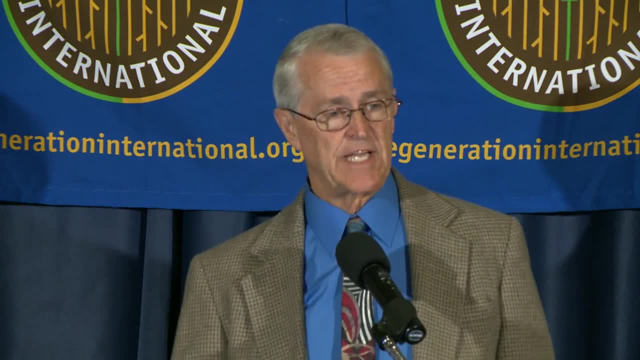 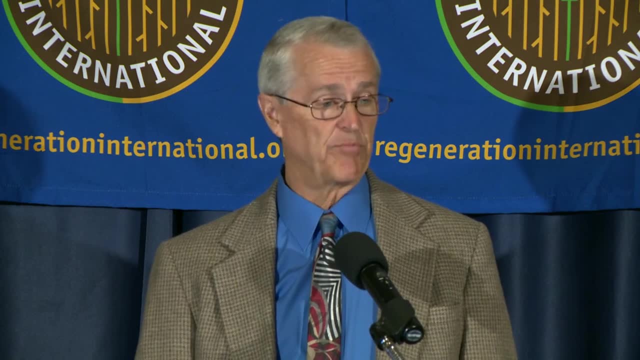 So farmers and ranchers will need to know that they will receive no less than a stable minimum price for their efforts, and businessmen will need to know that they will not be charged more than a maximum price for their investments so they can price it in to their products. 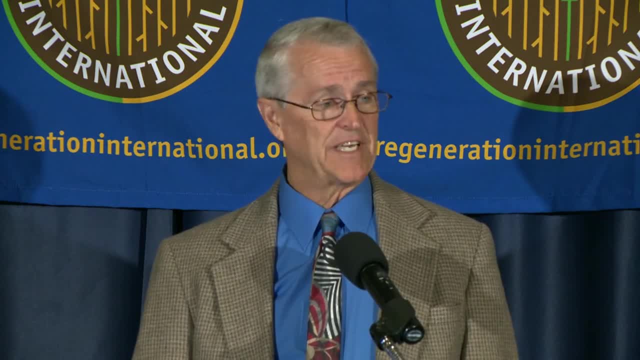 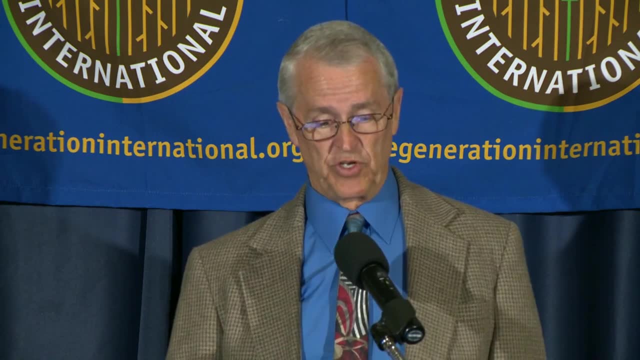 But most of all, the consumer needs to know that the money will be spent on the best system of emission reductions to remove or reduce atmospheric CO2.. This market could be available in EPA's Rule 111D. It requires mandatory 30% reduction. of electrical power plant emissions. It requires a reduction of CO2 emissions beginning in 2020.. Individual states and power companies are responsible and liable for these. Currently, the wording in Rule 111D does not allow carbon offsets in agro-ecosystems. But the Clean Air Act pretty much specifies that the reduction or elimination of the amount of air pollutants through any measures to protect and enhance the quality of the nation's air resources, to encourage and assist the development and operation of regional air pollution prevention and control programs. 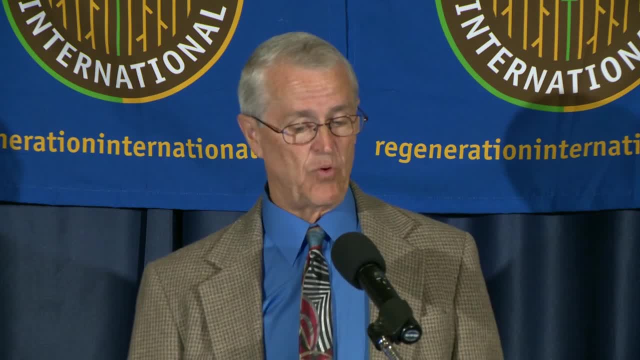 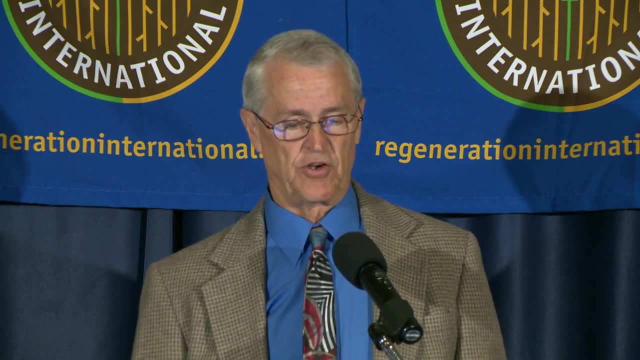 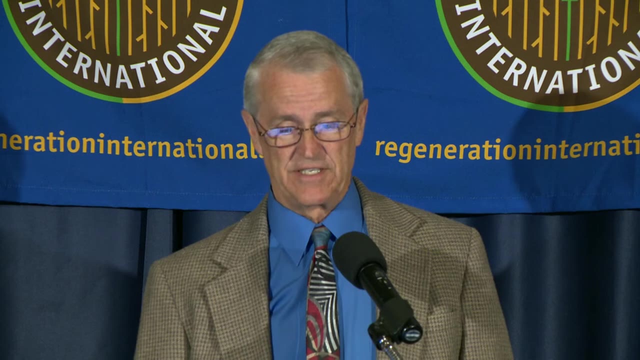 promote the coordination and acceleration of research, encourage and cooperate with institutions and organizations and individuals engaging in development and operation of regional air pollution prevention and control programs. Their criticism is that it deflects effort from abatement. But as Brian Murray from the Nicholas Institute said, 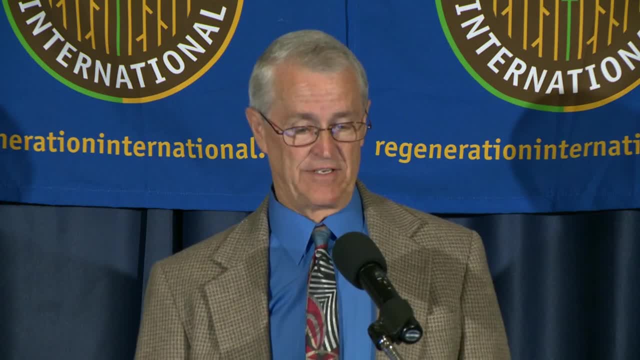 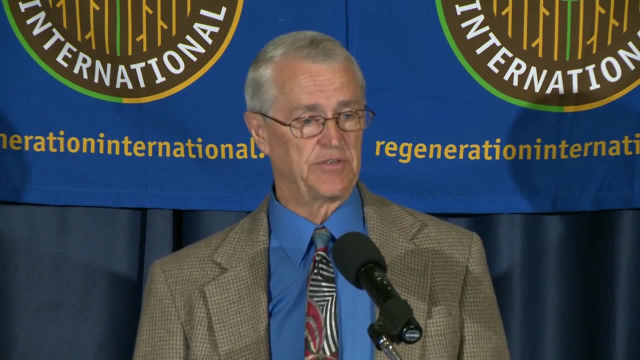 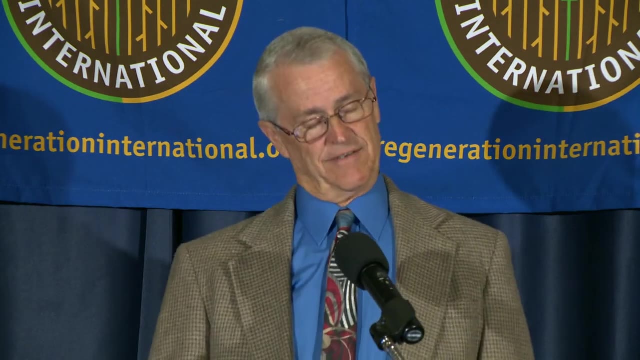 he said, in his view this criticism is misdirected. Deflecting abatement from cap sectors is exactly how offsets work. to reduce cost, It should be the overall reductions we are interested in, not where they occur. So the cost of CCS, which is EPA's recommended methodology. for reducing CO2, they only usually give you the CapEx cost and what it costs to build it. They don't give the financing, the parasitic loads, the overhead and maintenance and the transportation storage. As you can see, that price ranges from 218 to $264 per ton. of CO2. And they don't include any profit in there too, and I'm sure there's going to be a profit motive somewhere. If you compare renewables, most renewables are relatively expensive, from 58 to $377.. CCS- geological, as I said- 218 to 264.. 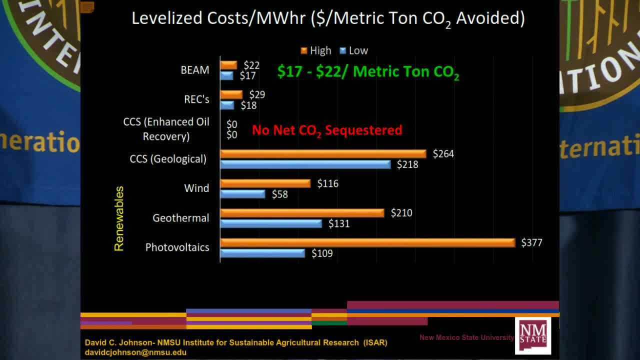 CCS- enhanced oil recovery. there's no net CO2 sequester. All that CO2 that's put back into a formation pushes oil out on the other end and you're burning that oil. you're just displacing where the CO2 is. RECs are the closest in price, but they depend on renewables, So the only system that we have is our agroecosystem using something like BEAM, and that price is from 17 to $22 per ton of CO2.. CCS, liabilities and geosequestration. 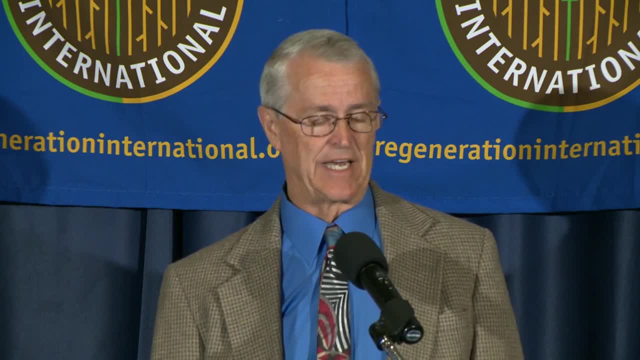 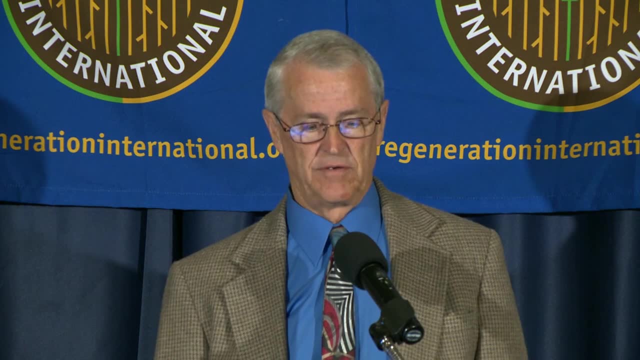 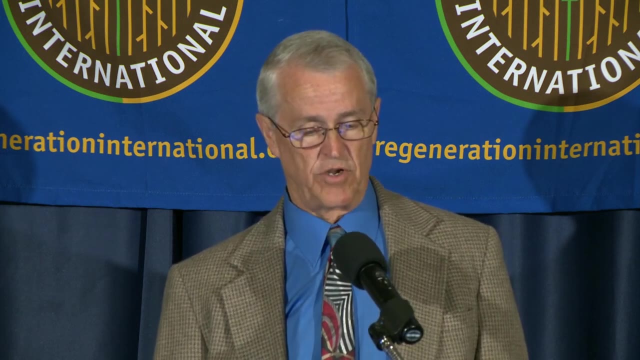 migration of injected CO2, unintended leaks, seismic activity, acidification of aquifers, long-term monitoring. no beneficial ecosystem services. whatever BEAM, however, gives ecosystem services that increase soil fertility, water storage in soils, plant water use efficiencies, soil nutrient availability. 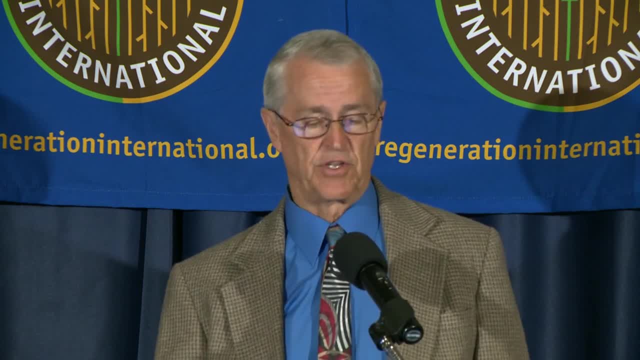 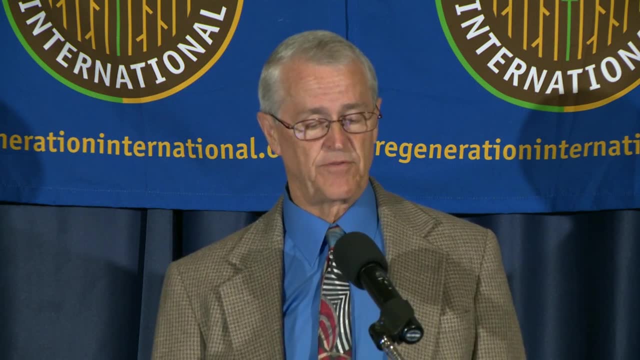 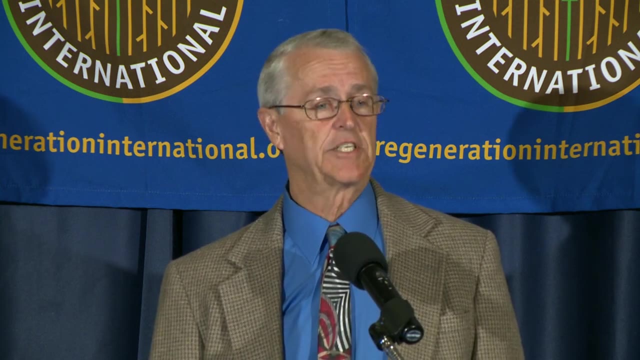 reduces plowing, reduces fertilizer application and downstream pollution of streams, lakes, rivers and coral reefs. It allows farmers to transition to a sustainable and ecosystem-friendly approach to agriculture too. Cost of offsets using ecosystems for carbon capture: a 6% energy surcharge. 1 cent per kilowatt hour increase in electricity, 15 to 17 cents increase in cost of gas and diesel, or $2.53 for the average plane flight- Less than the cost of a drink. We enjoy our lifestyles, but it takes energy to support them.